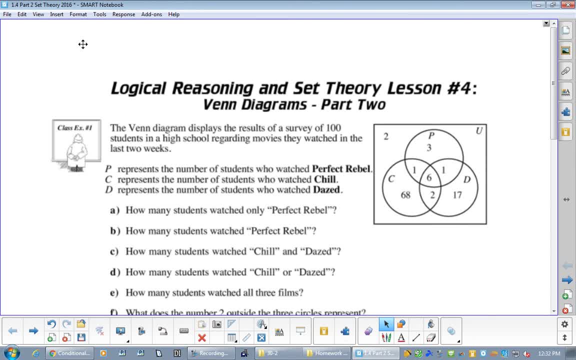 I've seen it many times Now: all we're gonna be doing today is really, really focusing on all the little nuances Again, all the specifics, all the language, all the little symbols, right. So it's kind of a review day. 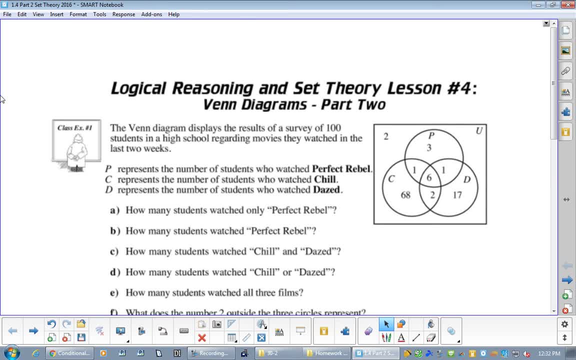 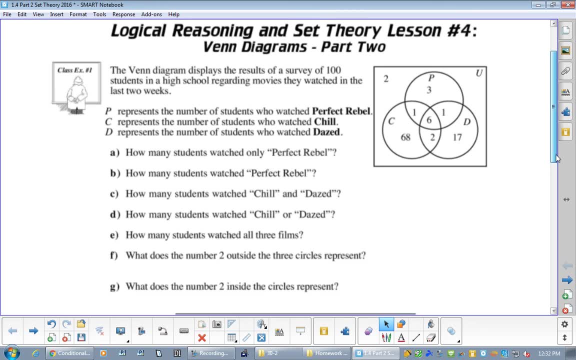 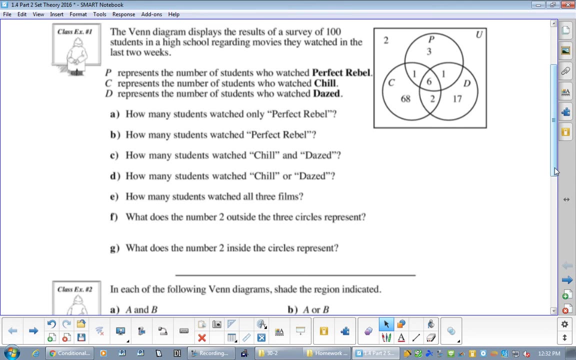 but asked in a different way. okay, Because I want, obviously, for you to build Venn diagrams. but what if this was the question and all they give you is a description which they will right? This is 100 students in a high school. 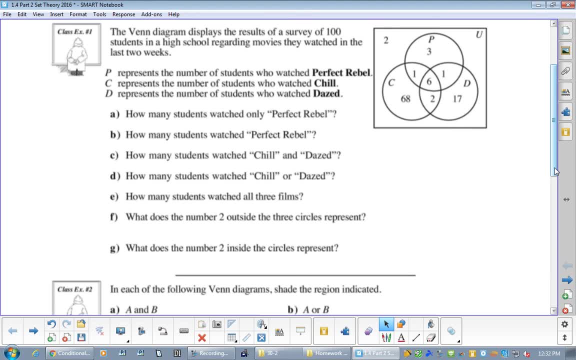 were asked regarding movies they watched in the last two weeks And of course these are not true names or else someone would get sued. So P represents a number of students who watched Perfect Rebel. C represents a number of students who watched Chill. 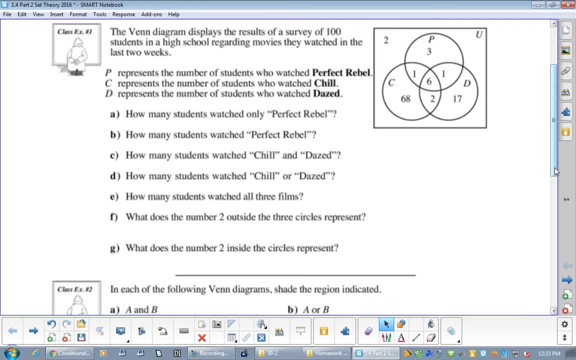 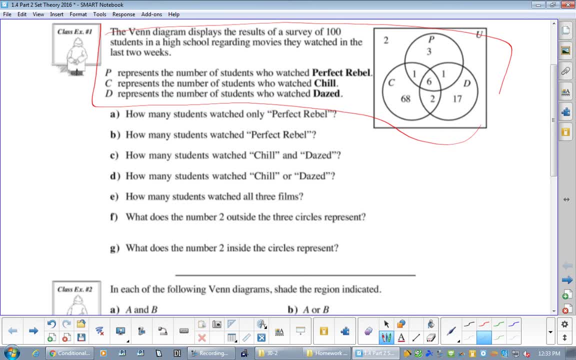 and they would just ask one of the following below: Okay, Now, just by looking at that number there, do we know what that means. What does it mean? They watched all three, okay, And is that? who can describe what that is? 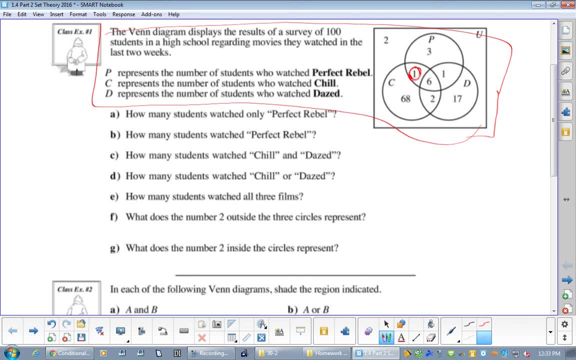 Okay, I need you to be specific with that. Say it again: Okay, so they watched Perfect Rebel and Chill but not Dazed. or they watched only Perfect Rebel and Chill, right, Like so. it's those little things and they're gonna have A, B, C, D. 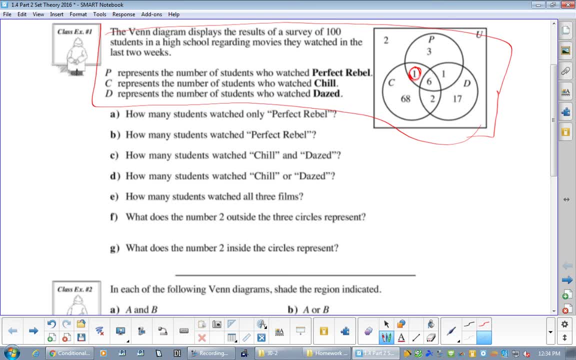 and you don't wanna be. ah crap, is it that one, or is it that one? Like? that's not a good place to be, And that's why I want you to be so definite with these Right. So all I want you to do right now 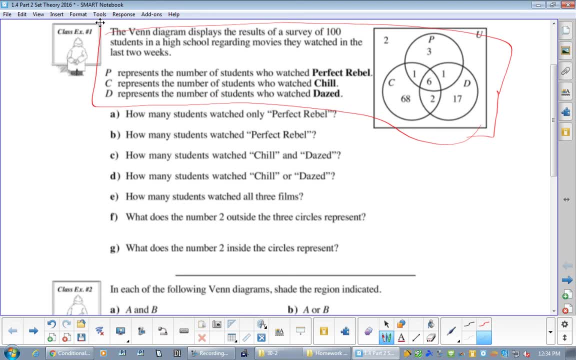 again. I'm just gonna pause the taping and it's fast. I just want you to do A to G. okay, Fill in the numbers if you get it wrong. Okay, so, as you read through these, you probably saw or you see: 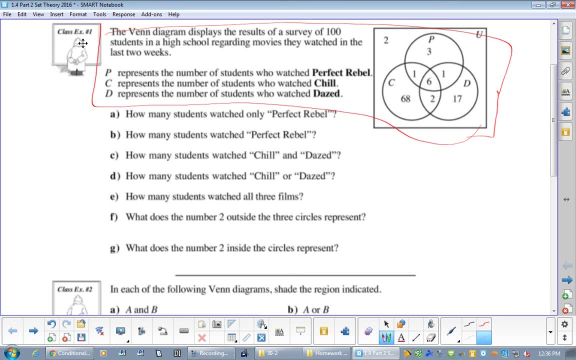 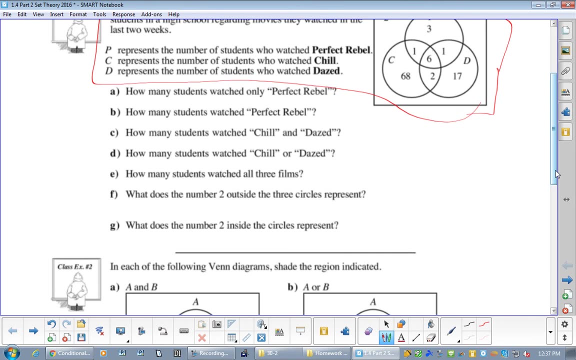 how they are trying to just change them a little bit to be able to mess with you. right, Because they're not giving away diploma marks. right, You do have to know the little nuances, or else, yeah, you will get them wrong. 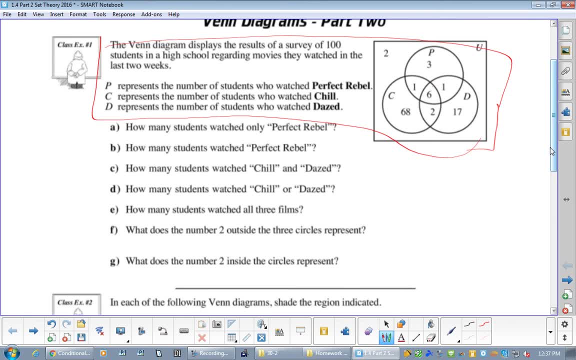 Now, obviously A and B would be conflicting. You do not want to wonder which one is which. So how many are we saying for A? Three, Three, How many for B? Eleven, Eleven, okay, So watched, perfect rebel. is all of these correct? 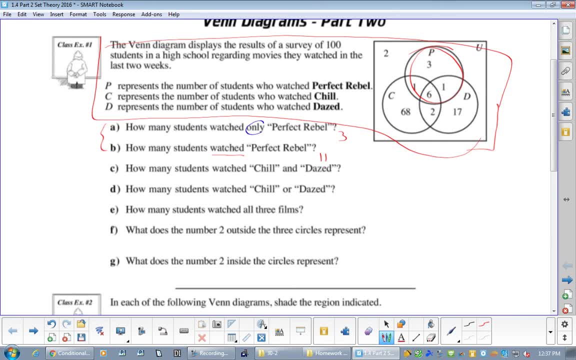 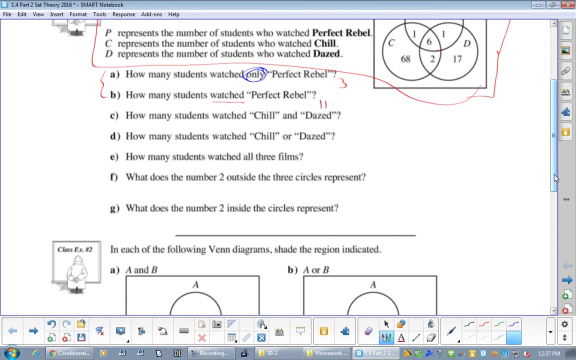 Okay, Watched, only perfect rebel would be just that one. That make sense. Okay, good, So I won't catch anybody on these. right, I won't catch anybody on the unit exam right Now. how many watched? chill and dazed. 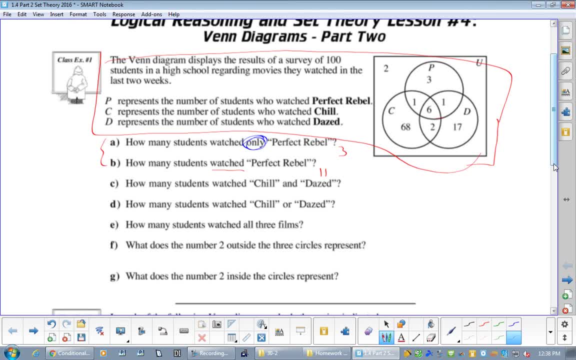 Okay, so we got people saying two and we've got people saying eight. Okay, let's figure it out. So how many students watched? chilled is obviously here and dazed is here. Okay, did these people watch? chilled and dazed? 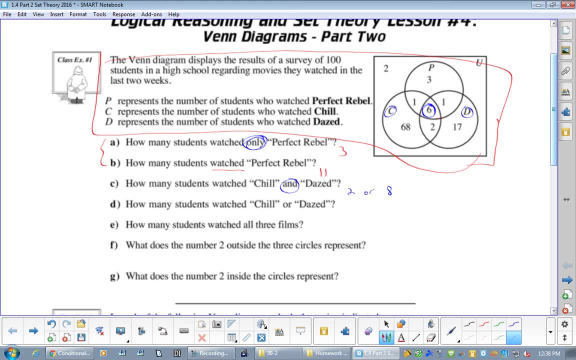 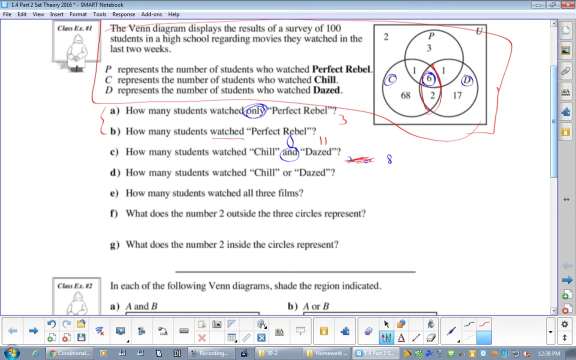 And usually means, Usually means the football, right? Okay, see, I'm glad we had this little talk. Better today than okay. So you can obviously see what kind of stuff I want on the course, i want on the quiz tomorrow too, to make sure you're getting these okay. so remember that we're 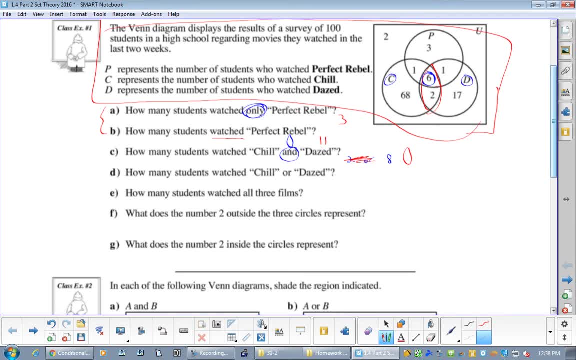 looking for the football, because six is part of those people that saw it. now i know they saw perfect rebel as well. i'm not saying they didn't, but they did see those two movies c and d. okay. now, how many people watched, chilled or dazed, how okay. what do we got? i heard a 95. what else? 87, okay. so here's another one that's gray, obviously. 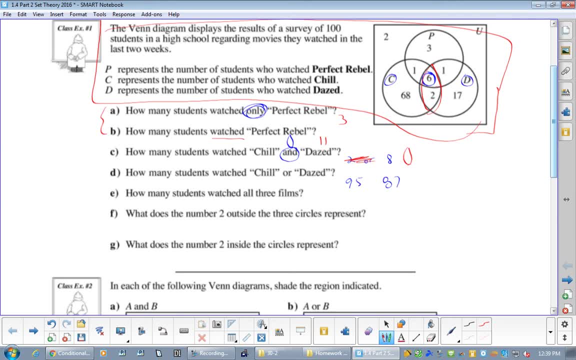 some people are: uh, so how many students watch chilled and dazed. i would assume we're talking this correct. yes, okay, now the 87. how did we get 87? did we forgot the six? that's still not enough. and the ones, right. so those people just did that. okay, so we want to. 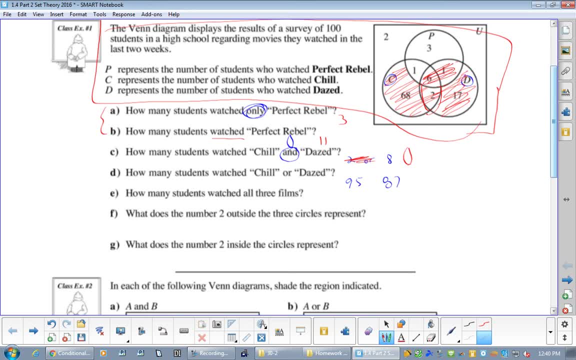 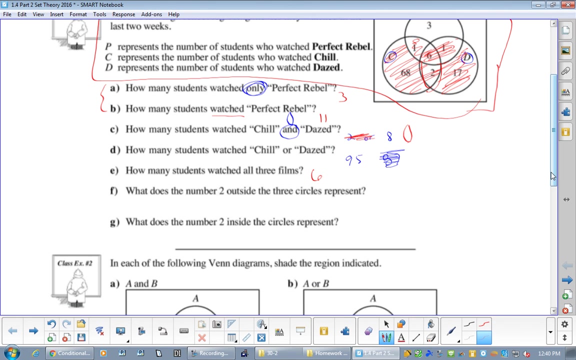 be really specific that these people too did watch it. okay. so again, yes, these can be tricky, okay. okay, how many students watched all three? okay, now, how many students watched perfect, reveled or chill or dazed? okay, so these people. what was the number two inside the circle? no movie, right? so what does the two outside represent? 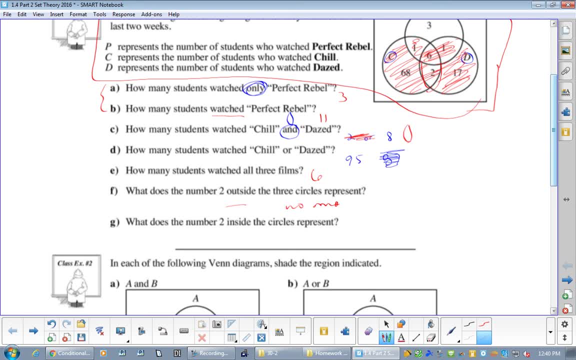 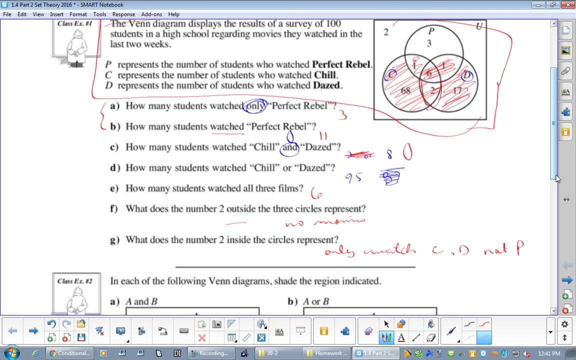 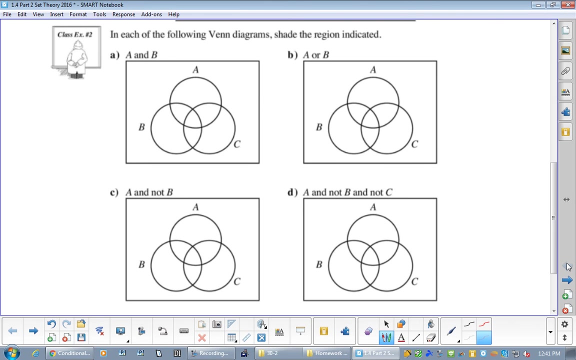 okay, no movies. what does the number two inside the circle represent? only watched, only watched C and D, not a, not P. yeah, okay, now again. all I want you to do is shade what they're talking about. okay again. okay, a and B. let's talk about that one first. 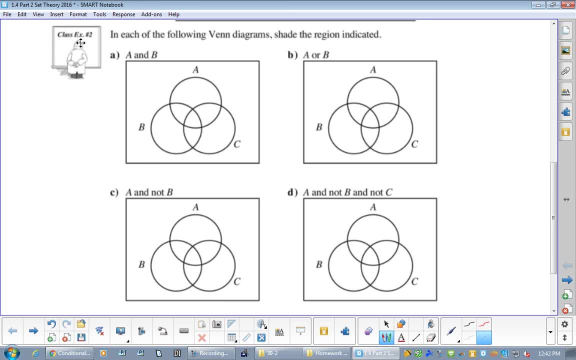 now, first of all, let's write this on top, because that's what that meant: a and B. what's the other way to say it? intersection B. yes, okay, so should be thinking football. so hopefully we shaded that a or B. how would I write that? a you okay? so please write the symbols above, because do not. what kind. 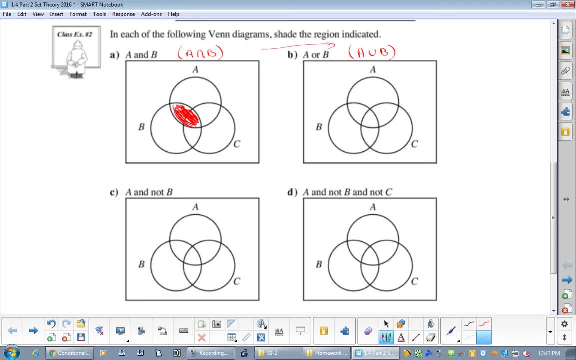 of psych say: do not, like we can't be at a test going crap. which one means? which? that for sure is, you're not ready. like you shouldn't have gone to the exam, you weren't ready for it. if you still don't know the difference between those two, 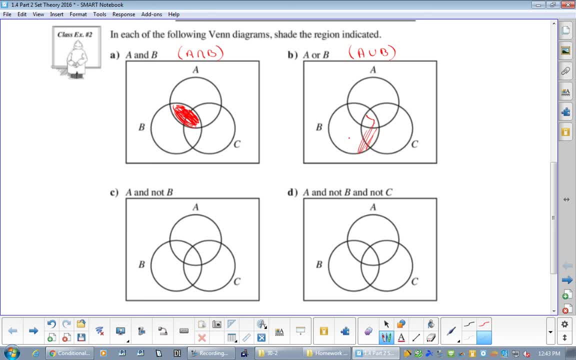 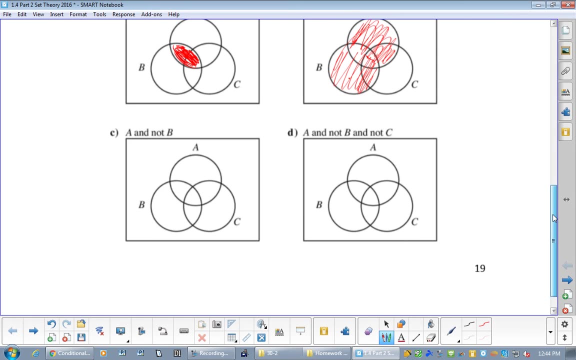 okay, and that one. you should have shaded that correct, okay. next one: a and not B. now we were doing it as a, not B. right, there's another way, because I was going through diplomas that they will say it will be a and not B. okay, a and not be. now that's the. 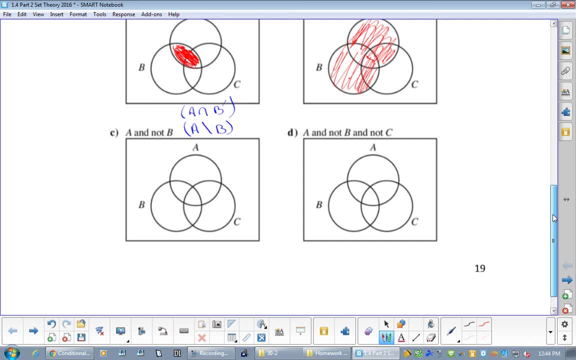 complement of B. but that means not B. right, it means everything but B. so a and not B. hopefully we didn't get into there and we're going to shade like that. okay, does that make sense? and the last one is a and not B and not C. now I've. 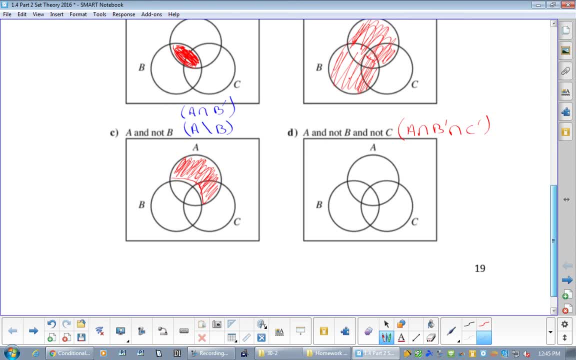 never seen the slash slash ever before. okay, I've seen it with the two: a not B. so this is the way it will probably be now: a and not B and not C means do not shade in any B, do not shade shade in any C. so hopefully we got that okay. so again, just being really careful that we're going. 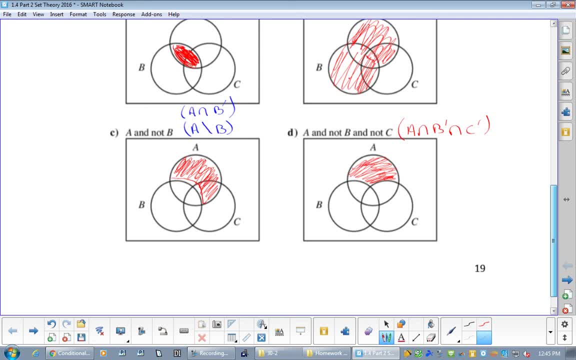 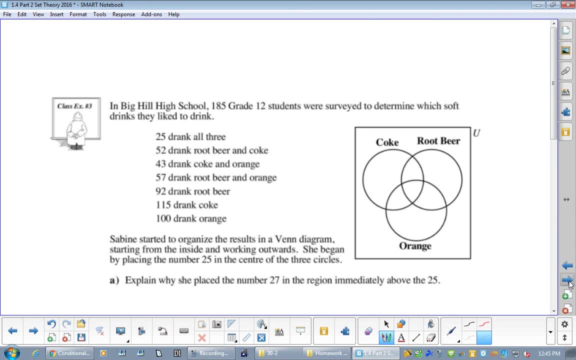 over this again and make sure everybody gets it. okay now the other is: if they just get in the middle of the line and they don't get in the middle of the line, and they don't get in the middle of the line and they don't get in the middle. 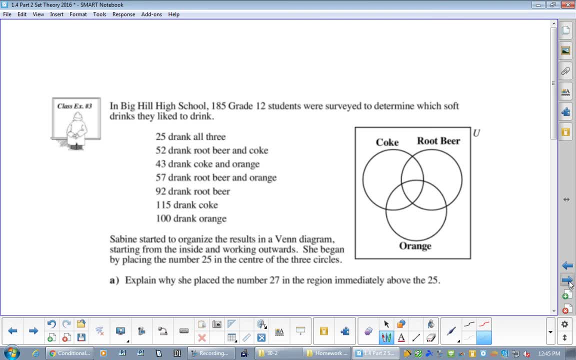 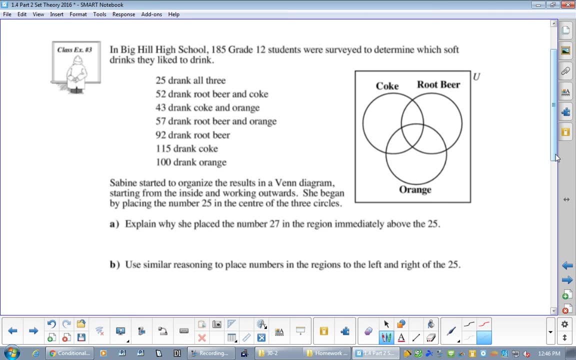 give you the numbers and you have to come up with the entire Venn diagram. so, again, I just want to. I'm going to pause tape- see if you can make this Venn diagram, and what you want to do is look for the for sure's like this one, right? 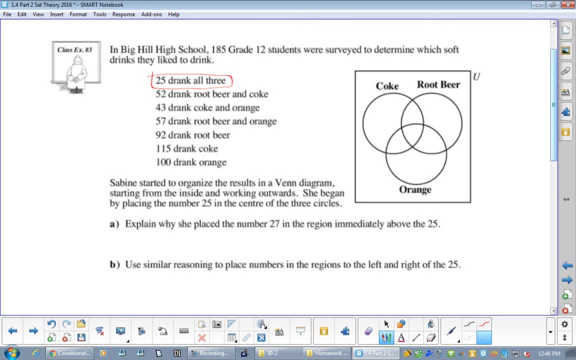 here. that's money, right, everybody knows where that one should go. that's our middle. that helps a lot. and then you got ands- what a hands represents. so this is your middle, what a hands represent. yeah, what a hands always represent. yeah, that's my footballs, right, like I want you to remembering those. 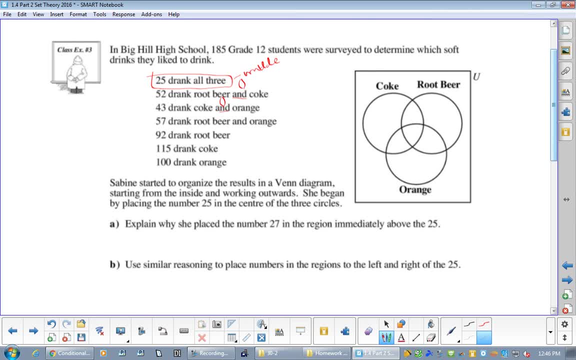 stupid cheesy things when you're in the diploma, right, it trust me, you just feel like I got this one okay. seen it a million times. done this one okay, so just see if you can fit it. fill this in quick. should take you about two minutes. so let's see if you got this now. first of all, your middle should be 25 and then 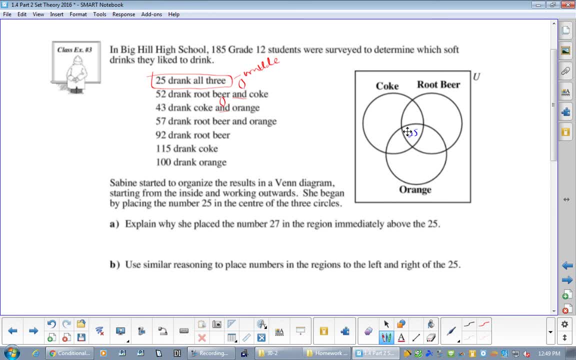 it said 52 drink, root beer and coke. so my football I'm gonna go 52 minus 25 and I should get 27 there. those two together should equal 52, which they do cross it out, maybe because I already did it- 43: coke and orange, coke and orange. so 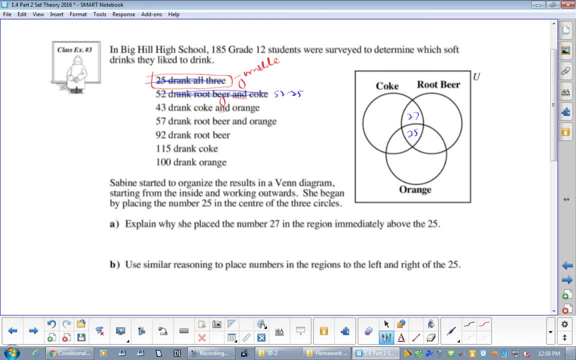 that's that one. so 25, 43 minus 25, I should get 18 there. then my last football is 57 drink root beer and orange, so these two equal 57. right, so far, so good. okay, now it said 92 drink root beer, so my entire root beer should. 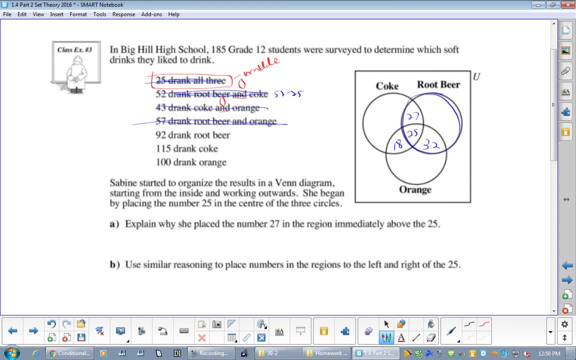 equal 92. 27 plus 25 plus 32 minus 92 gives me eight. right then I'm going to coke 115, right? so 115 minus 27 minus 25 minus 18 should give me 45, 25,. okay then. the last one is orange. I'm going to go minus 18, 100 minus 18 minus 25. 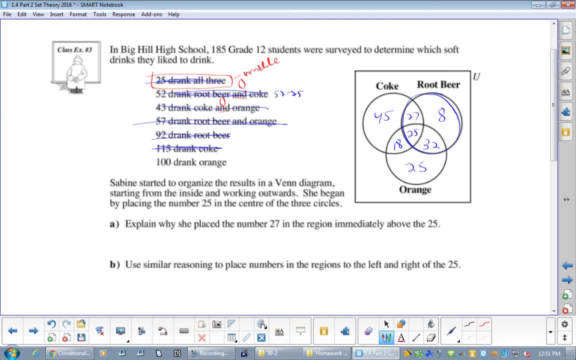 minus 32, and I got 25,. right, what's that? that only equals 180,. so some people I said you weren't totally done, you needed that 5 there again subtle, but a killer, remember on the quiz, if we left that out, you're like: is it wrong? and I'm like: oh yes, it should. 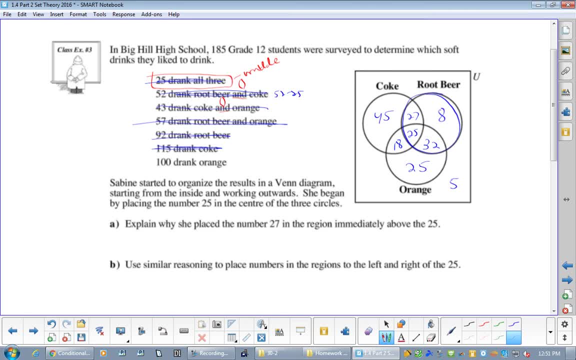 be wrong, but I forgot to look at it when I was coming around. but okay, so right. so this all equals 180, right, but it said 185.. Therefore, remember, our universal set must include everybody. okay, so this is like: 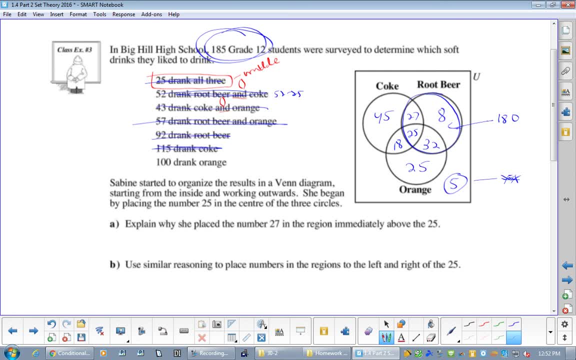 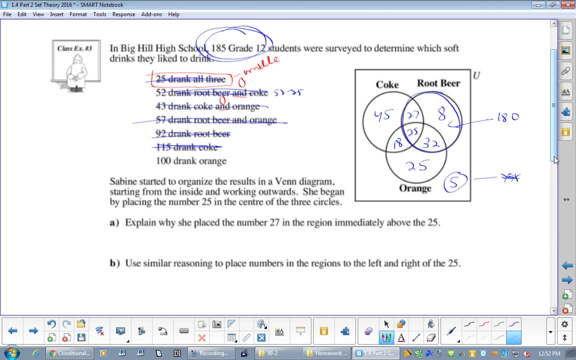 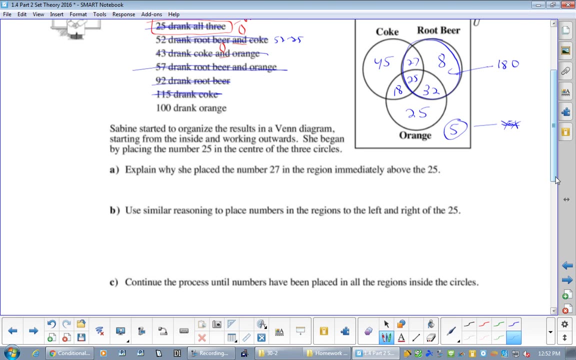 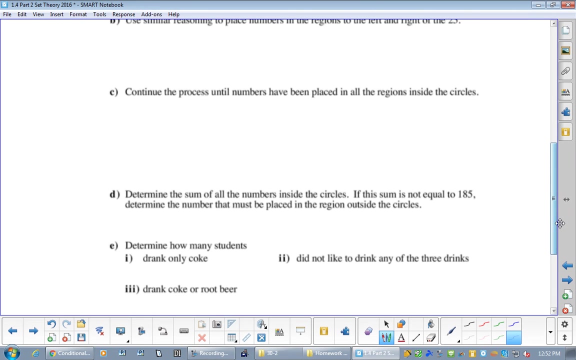 okay. so all of these questions below are the same things as above it used. you know, if we don't, how many students drank only coke? okay, we should be saying 45. how many did not like any of the drinks? 5 and the excellence diploma question? I think will. 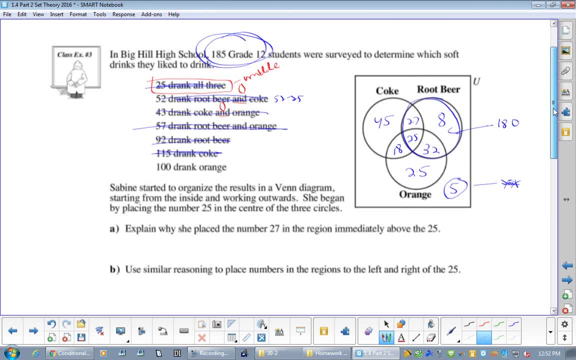 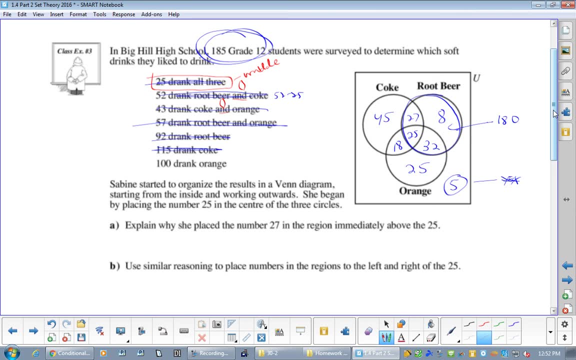 be this one, because they'll give you all of this and they'll say how many people did not like any of the drinks. they will not have the five there, just like I didn't have the five there, right, but that would be an excellence question. okay, so that's what I say. excellence like it. that's their nine ten out of ten. 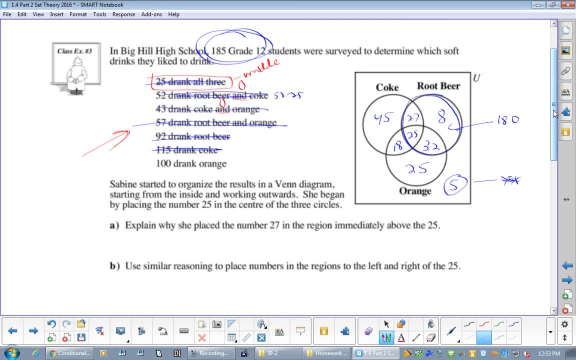 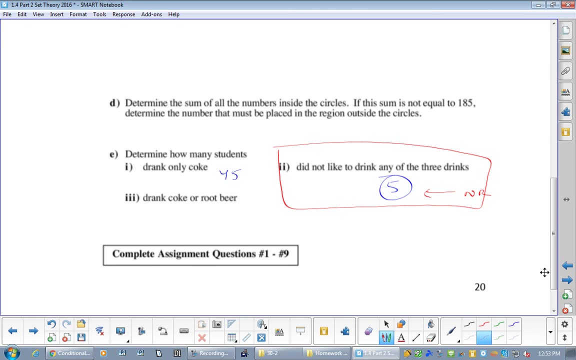 difficulty? is it impossible? no, is it a bit of work and do you have to know a lot of stuff to do it. that's why they call an excellence question. right, that would? this would be what I was. that's an a numerical response question, right there. right, you just put a five in and you're done, right, but it takes probably. 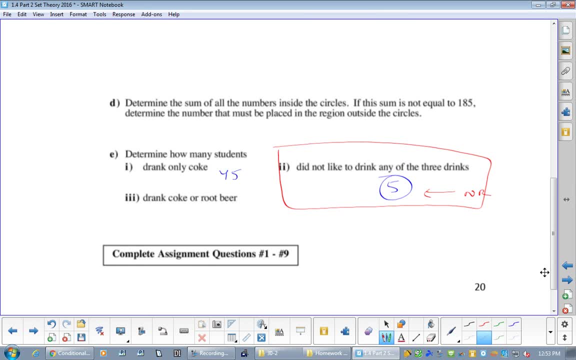 three, four minutes to get to that five and they're unnerving because, like, I hope it's five, did you get five? that's what you mean. when you walk out you're gonna like: did you get five for that one? yes, you don't want to talk to anybody else. right, I got what I needed to know. I. 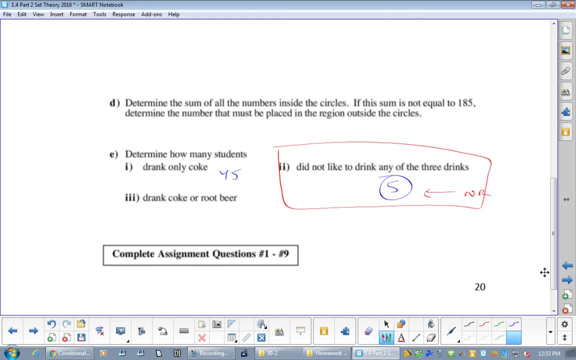 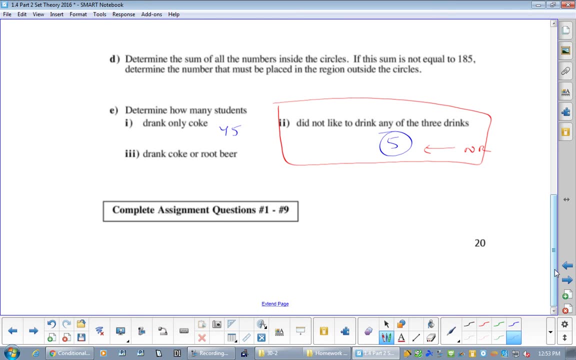 do not want to hear that six or four from anybody else, I'm happy. yeah, it's when. it's when one guy's got six and other people have five and you guys like trying to convince everybody they're wrong. well, it might be you I've had- I don't know how many students I know have- 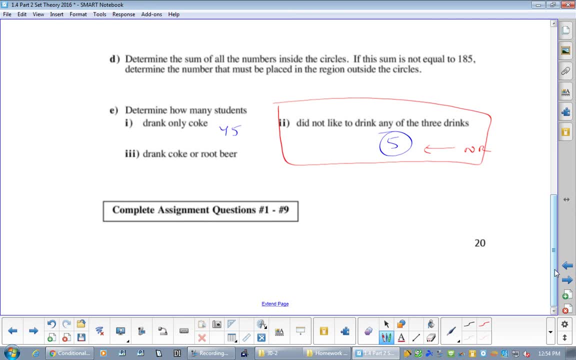 marked their diploma when they've come out, like I had a girl going in with a hundred and when I talked to her the next day or no, an hour later she goes. I got one wrong. yeah, she knew right, because everybody talks right and yeah, I mean it sucks, but she knew right. yeah, I got one wrong and she did, she got.